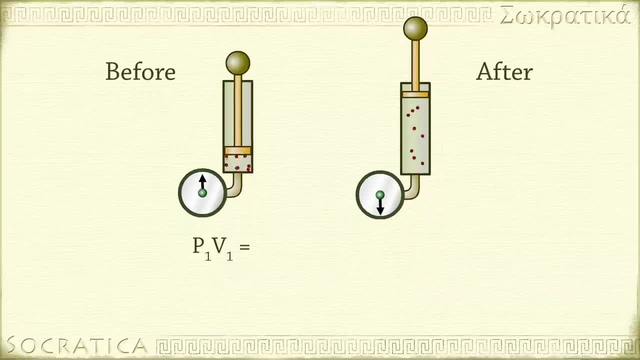 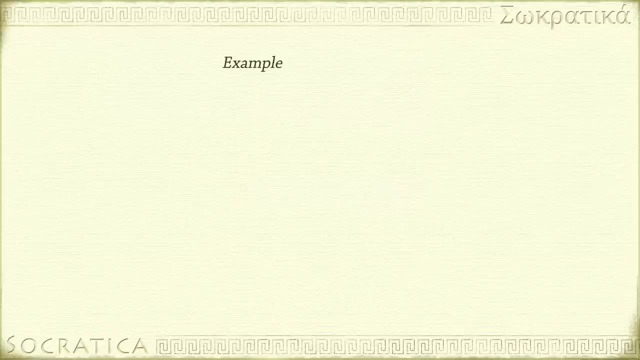 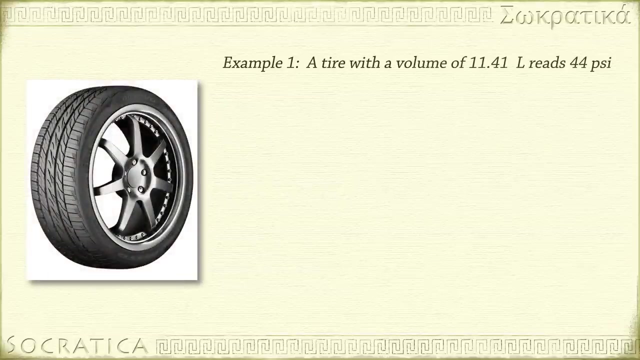 that case you can say P1V1 equals K and P2V2 equals K. so you can write Boyle's law as P1V1 equals P2V2.. Let's see an example. A tire with a volume of 11.41 liters reads 44 psi on the tire gauge. What? 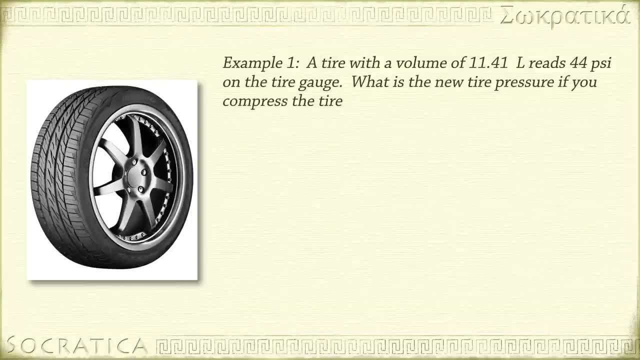 is the new tire pressure And its new volume is 10.6 liters. Write out Boyle's law and substitute in what we know. This is one of those before and after situations. so we write: P1V1 equals P2V2.. 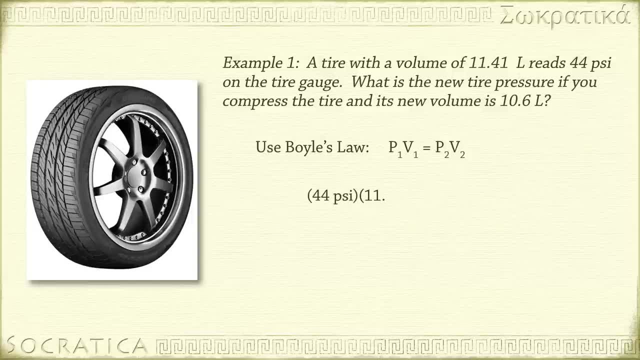 44 psi times 11.41 liters equals P2 times 10.6 liters. Solve for P2.. Divide both sides by 10.6 liters. 44 psi times 11.41 liters equals 10.6 liters. Solve for P2.. Divide both sides by 10.6 liters. 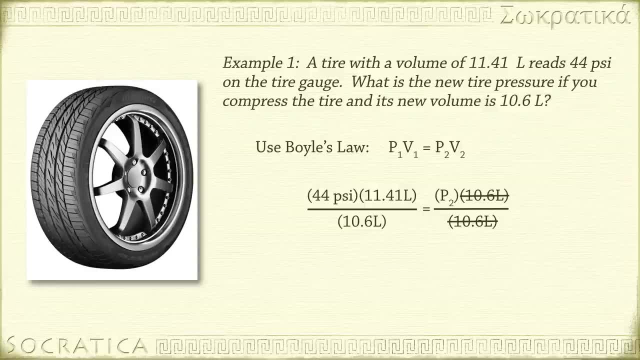 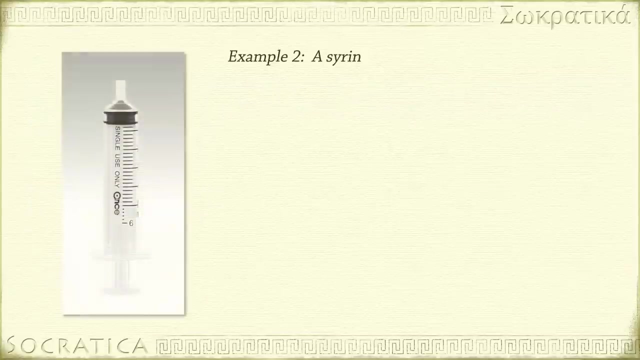 P2 относ to P2 equals 47.36 psi. There are two significant figures in the measurement 44 psi, so we round our answer to two sig flecks – 47 psi. Here's another example: A syringe has a volume of 10.0 cc's – or 10 cubic centimeters. 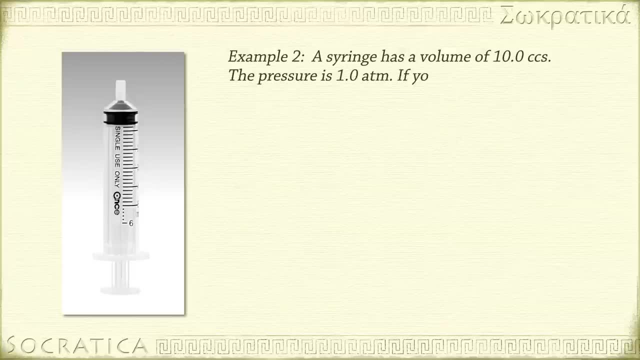 The pressure is 1.0 atm. If you plug the end so no gas can escape, and push the plunger down, what must the final volume be to change the pressure to 3.5 atm? P1 V1 equals P2 V2.. 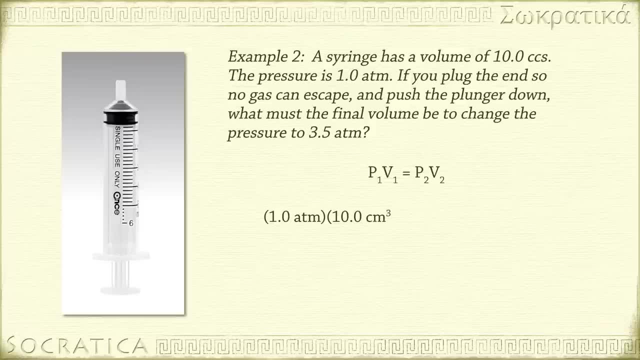 1.0 atm times 10.0 cm3 equals 3.5 atm times V2.. Solve for V2.. Divide both sides by 3.5 atm. 1.0 atm times 10.0 cm3 divided by 3.5 atm equals V2.. 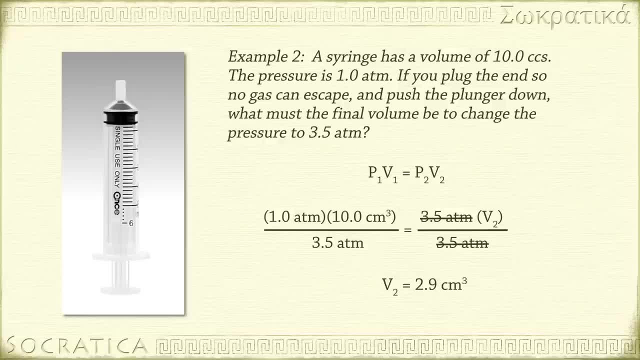 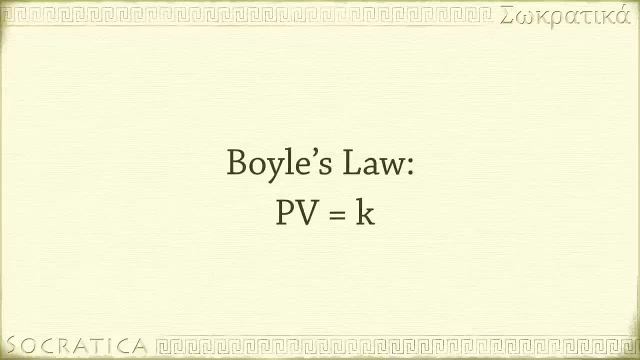 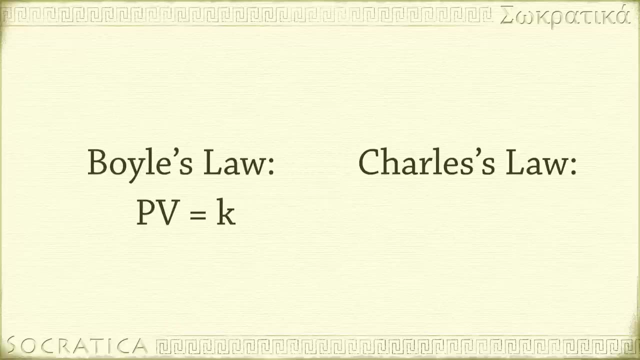 V2 equals 2.9 cm3, or 2.9 cc. Boyle's law relates pressure and volume, but there are other gas laws which relate the other essential variables associated with a gas. Charles' law is the relationship between the pressure and volume.